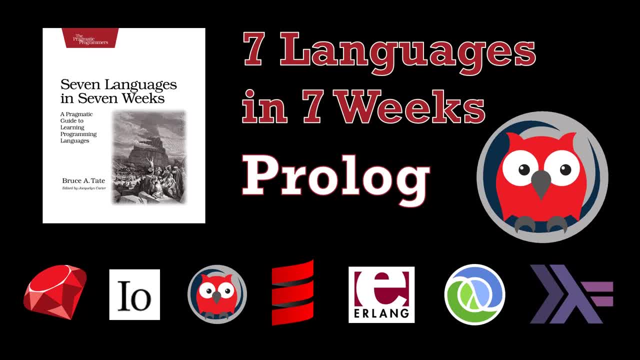 Welcome to a programming languages virtual meetup. pre-recording. My name is Connor Hoekstra and in today's video we're going to be covering chapter four of seven languages in seven weeks by Bruce Tate, and the third of seven languages, and today's language is prologue. Looking at the table of: 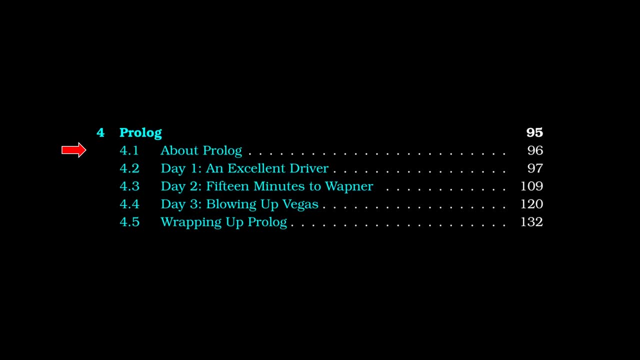 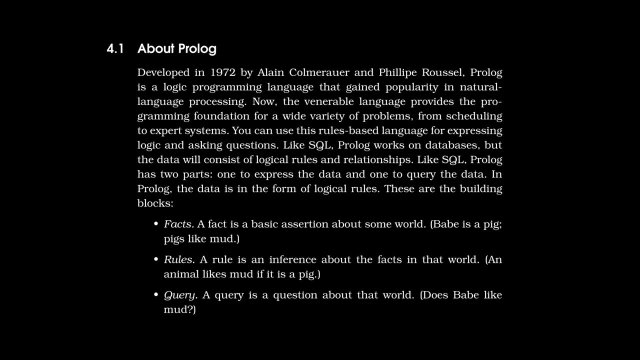 contents, which is the same basically for every single language chapter. there is an introductory section, a wrap-up section and then three days. So, hopping into the introduction section, the text reads: developed in 1972 by Alan Komarar and Philip Roussel. Prologue is a logic programming. 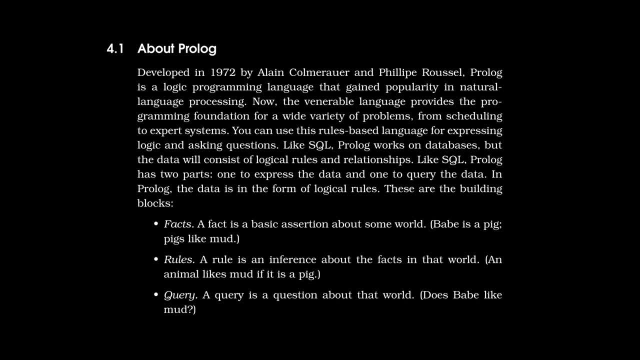 language that gained popularity in natural language processing. Now the venerable language provides the programming foundation for a wide variety of problems, from scheduling to expert systems. You can use this rules-based language for expressing logic and asking questions like SQL. Prologue works on databases, but the data will consist of logical rules and relationships, Like 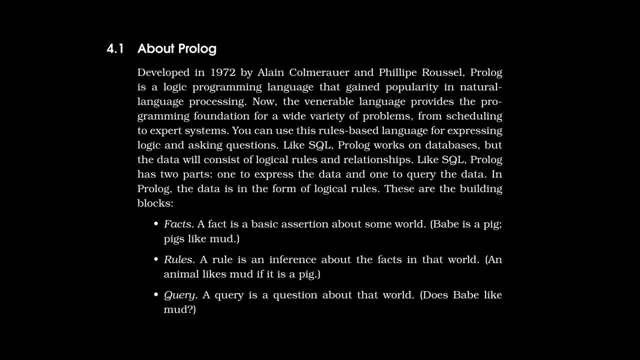 SQL Prologue has two parts: one to express the data and one to query. the data Prologue is a language that is used to express the data and one to query. the data Prologue is a language that is used to express the data and one to query. the data Prologue is a. 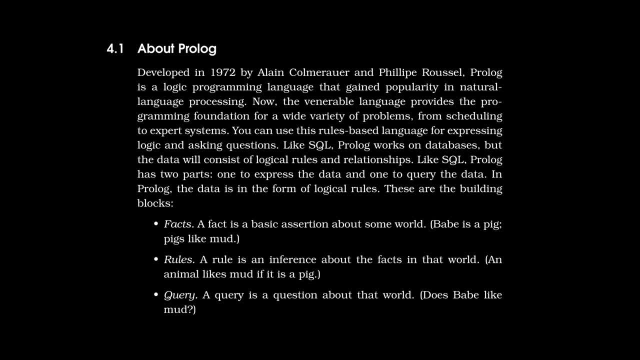 language that is used to express the data and one to query the data. In Prologue, the data is the form of logical rules. These are the building blocks. Facts: a fact is a basic assertion about some world. babe is a pig. pigs like mud. Rules: a rule is an inference about the facts in that world. 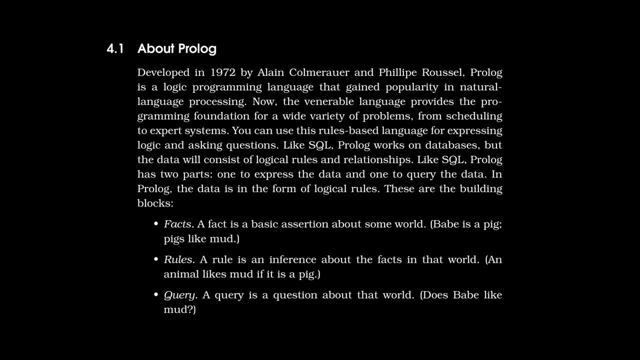 an animal likes mud if it is a pig And a query? a query is a question about the world- does babe like mud? And if we take a look at the programming language dependency graph that we generated for the previous video on IO, you can see that Prologue sits. 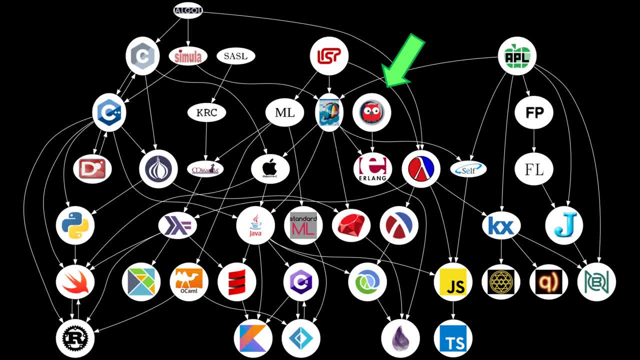 close to the top of the diagram where the little owl logo is. So this is the logo of SWI Prologue, which is an implementation of Prologue, And, interestingly, you'll note that there are no languages that Prologue is dependent on, because Prologue was the language that basically defined. 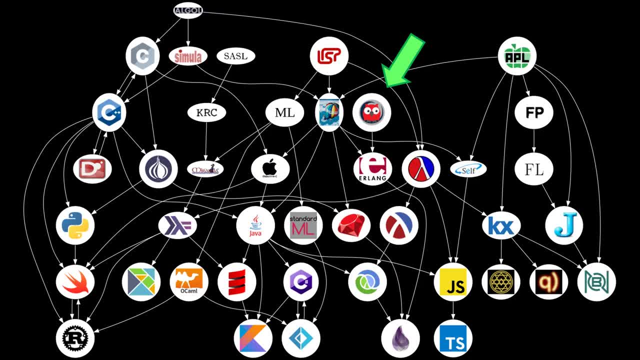 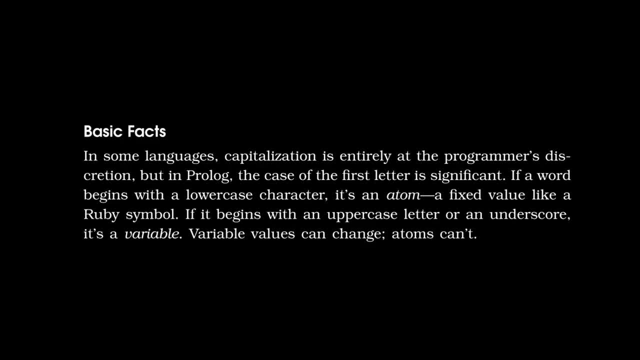 the logic programming paradigm. Hopping into day one of looking at Prologue, the first thing we're going to look at from the text is the section entitled Basic Facts. So it says in some languages capitalization is entitled Basic Facts. So it says in some languages capitalization is entitled 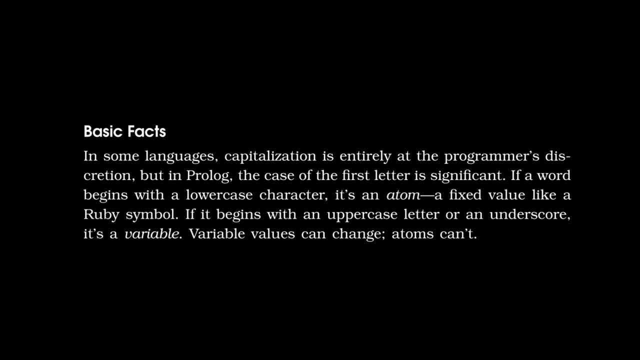 at the programmer's discretion. But in Prologue the case of the first letter is significant. If a word begins with a lowercase character, it's an atom, a fixed value, like a ruby symbol. If it begins with an uppercase letter or an underscore, it's a variable. Variable values can change. 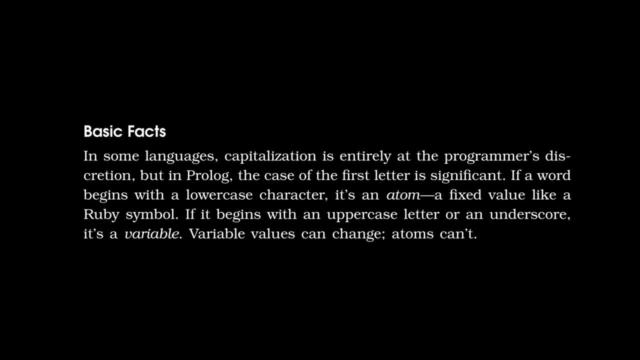 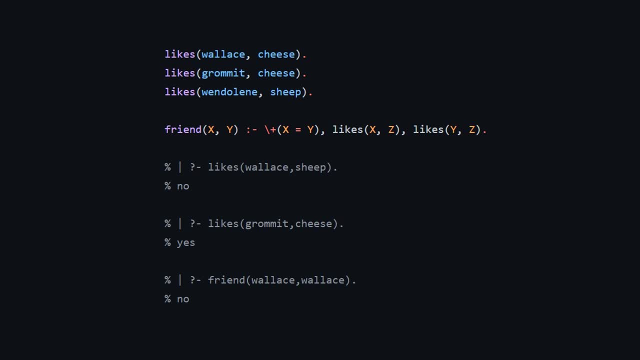 atoms can't. And so now we're going to look at our first piece of code from the textbook, which is an example stolen from the Wallace and Gromit comics, And here it says three assertions: that Wallace likes cheese, Gromit likes cheese and Wendy likes cheese. So we're going to look at 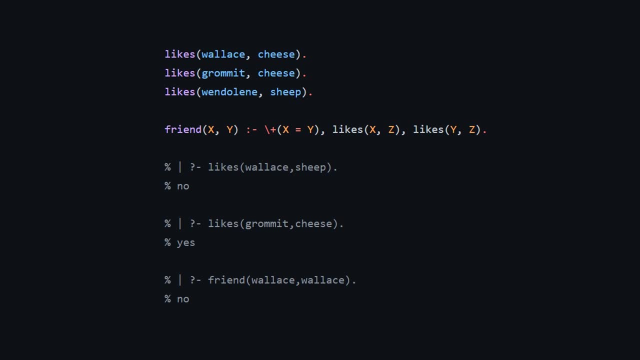 the first one. And then we have a friend rule that says for x and y, colon hyphen, which is sort of the assertions that are going to come after the rule x equals y, except it's preceded by a slash plus, which means not, So x does not equal y, and x likes z and y likes z, So it's. 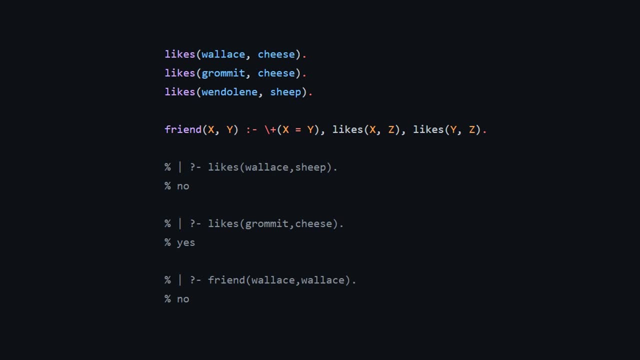 basically saying if two different entities both like z, then they're considered friends. And then you can ask the Prologue queries: likes Wallace sheep, is that true? It'll say no. Likes Gromit cheese? that's yes. And then you can. 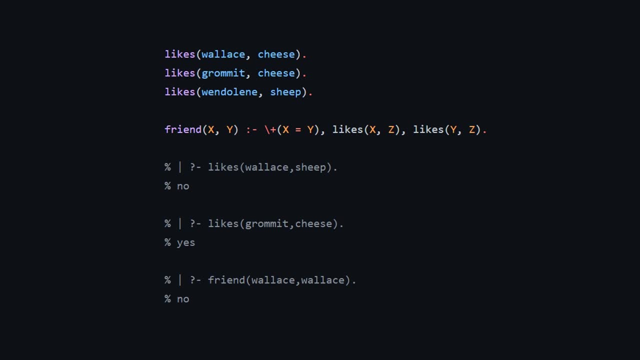 ask: is Wallace friends with Wallace? Well, they can't be equal to each other. But if you were to ask, is Wallace friends with Gromit, it would return yes. So that's our first example, And this is followed up by a second example which uses variables. So currently we only have 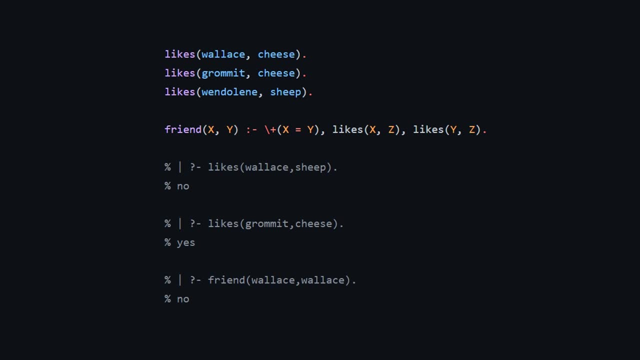 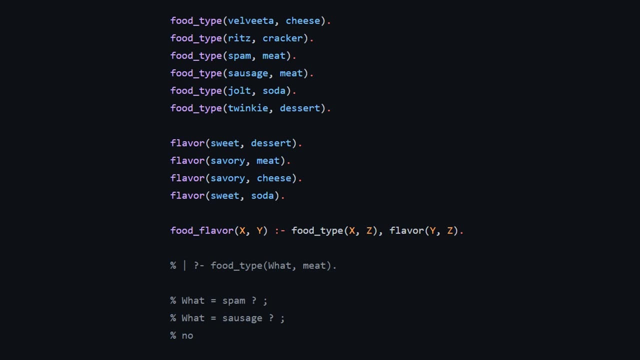 lowercase atoms and assertions and rules. But in the next example we also have a capital lettered variable. So this is a bunch of different foods with sort of flavors and the type. So we have food type and flavor And then we have a food flavor is: 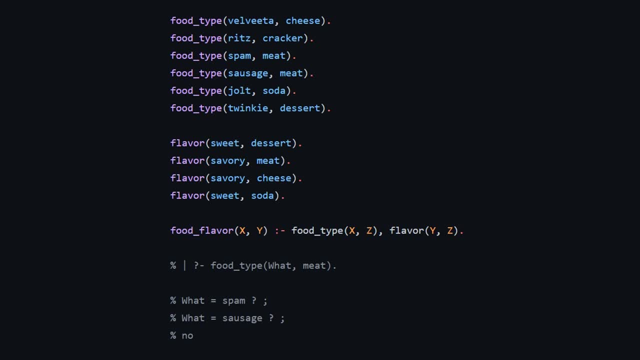 basically saying: given a food type, x and z return. you know the flavor, y and z, So you can get the food flavor using this rule. And so at the bottom you can see, we're just querying what are the different types of food that qualify as meats, And we do this by using a capital W'd. what in the? 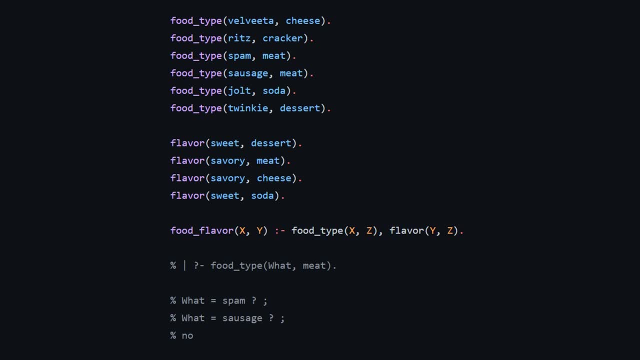 position where the type of food would be. So you can see that it returns spam and sausage. And note that when you're interacting with prologue in the command line, the semicolon is how you get the next answer And then, once there's no more answers, it'll return you a no. Moving on to the third, 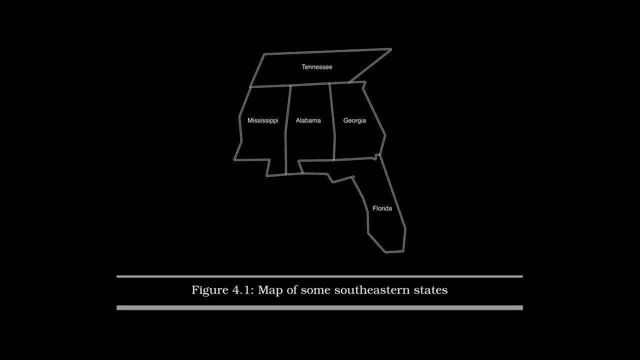 example that we're going to look at in day one. this is probably the most interesting one, And it's basically a map of five different states in the United States of America: Tennessee, Mississippi, Alabama, Georgia and Florida. And this is the map coloring problem, where they don't. 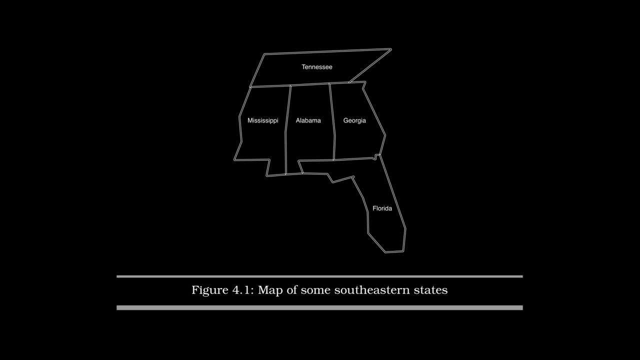 want any two adjacent states to have the same color, which is typical of what you would find in a map. You don't want bordering countries to have the same color, or bordering states, And the way that you can solve this is pretty simple in a logic programming language like prologue. So you 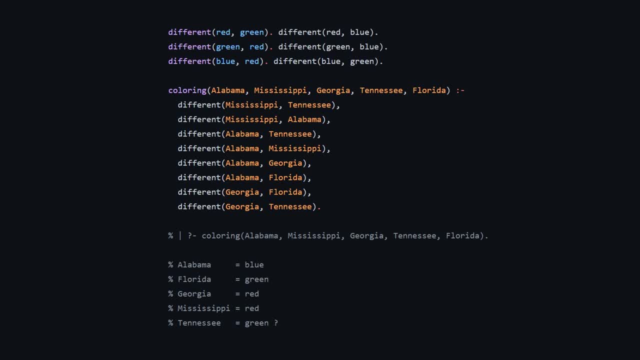 set up six different, different rules that the colors red and green are different, and then all the other colors are different, And then you set up a coloring of the five different states and you want each of the states that are bordering each other to have different colors. So you basically: 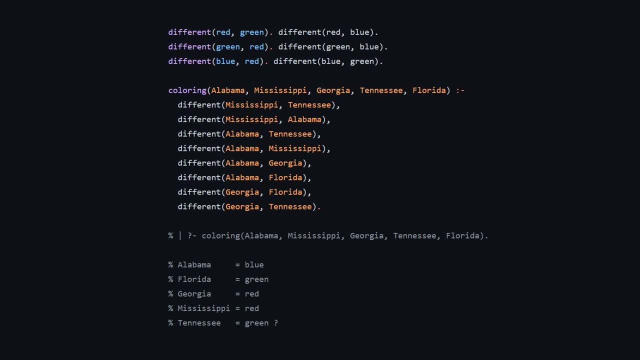 pass on the states to different And then, when you query coloring, you set up a coloring that has different colors, And then, when you query coloring for the five states, you end up with Alabama equal to blue, Florida equal to green, Georgia equal to red, Mississippi equal to red, and. 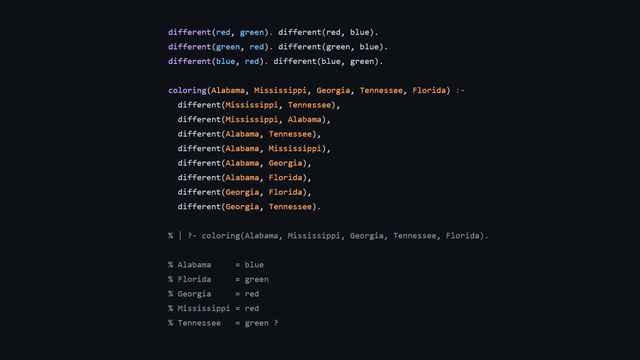 Tennessee equal to green, And I'm not sure if there was multiple solutions, because I just copied this from the textbook, But supposedly if you had hit semicolon you would have been able to get an alternate coloring, if it existed, And obviously there would be other solutions because you could. 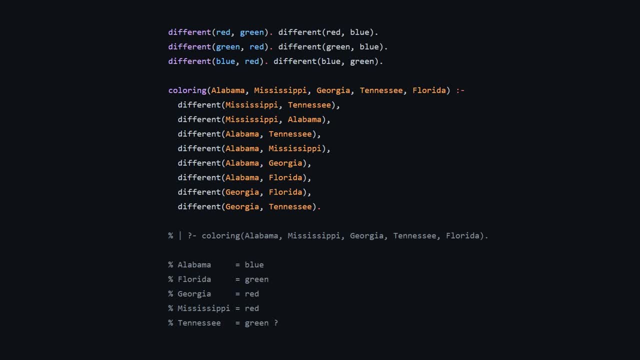 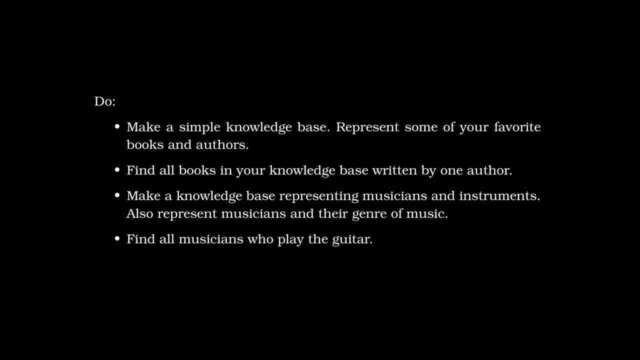 just basically permute the colors such that you have the same. you know, red is replaced by blue and it would have the same effect. And moving on to the exercise section of day one, it basically asks you to come up with your own knowledge base. So create some assertions on your own, based on 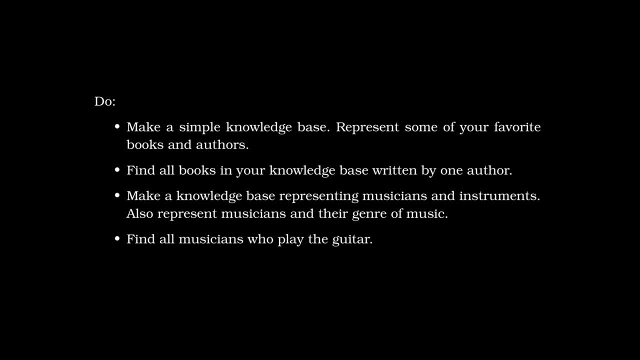 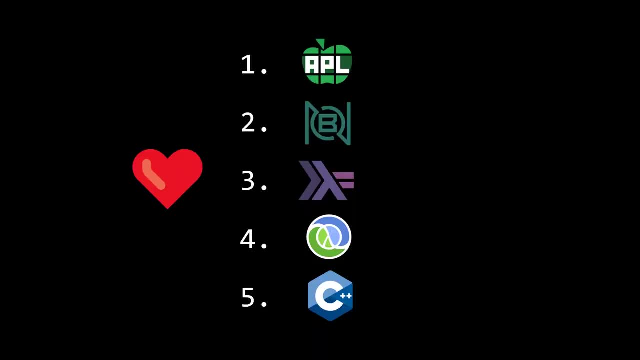 books and authors and then to write some queries. I decided to do this with programming languages because this is the programming language virtual meetup, and decided to do it based on my five favorite programming languages. So the last time that I actually stated my five favorite languages- 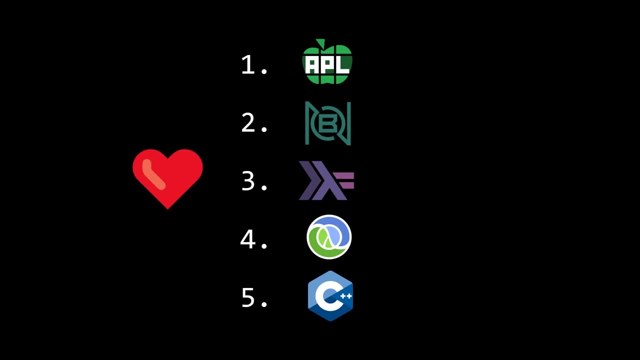 was in my functional versus array programming talk, which I will link to in the description below. So if you have any questions, feel free to reach out to me and I'll be happy to answer them. And if you have any questions, feel free to reach out to me and I'll be happy to answer them. And if you 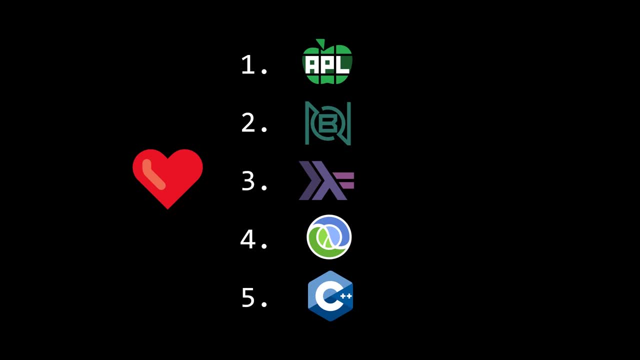 the description and in the top right hand corner, if you want to go watch that. And that was, I think, in October of 2021.. It is now March of 2022. And I would say BQN at this point is my favorite. 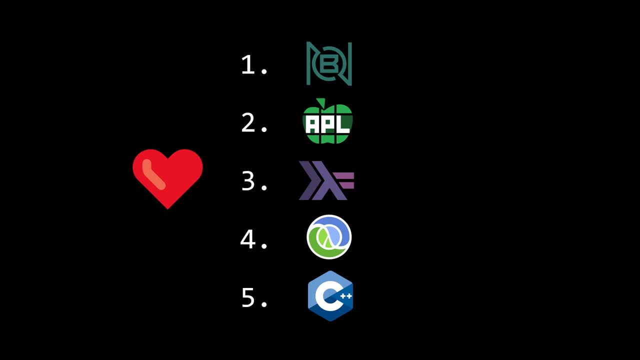 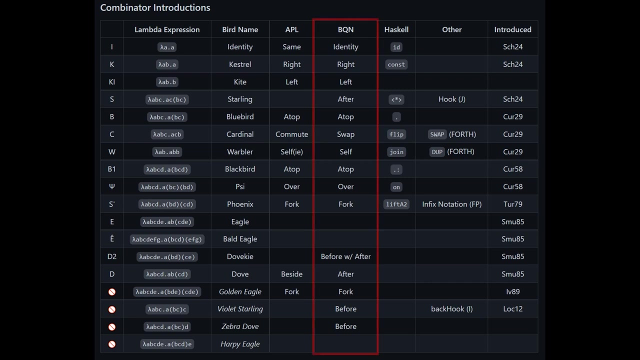 language. BQN is basically the next generation APL and takes influences from other languages like J, And the reason for this is because BQN is a more powerful combinator language than APL is. If you take a look at this combinator table that I drew up, you can see in the middle. 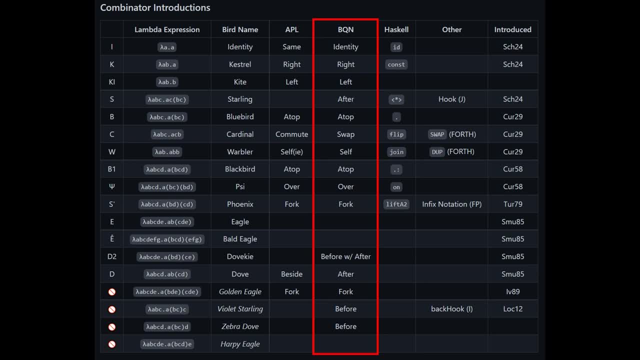 BQN has more support for different combinators from combinatory logic, And you'll note that APL, BQN and Haskell are all on this table and they correspond to my three favorite languages, So combinators are a reason why I love these languages. There are other reasons as well, but 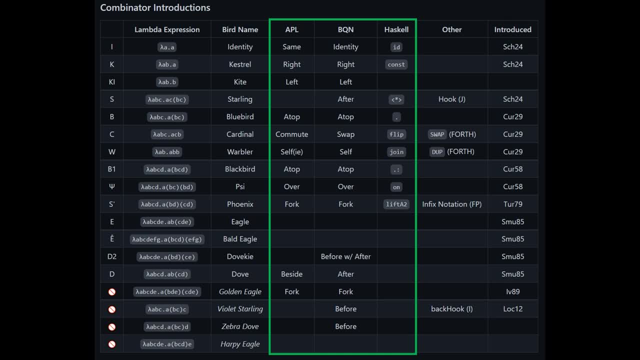 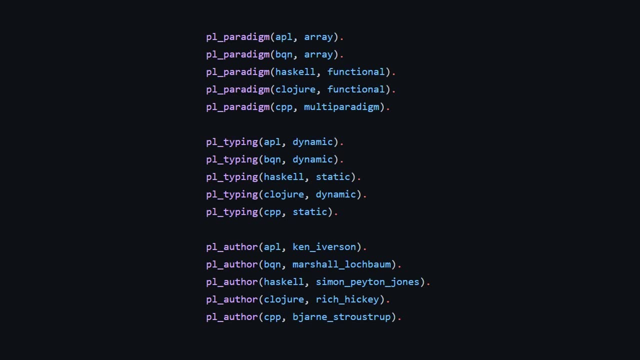 I will give a future talk on combinators and combinatory logic at some point. With this in mind, we can build our little knowledge base with assertions. So we have different paradigms: array for APL and BQN, functional for Haskell and Clojure. 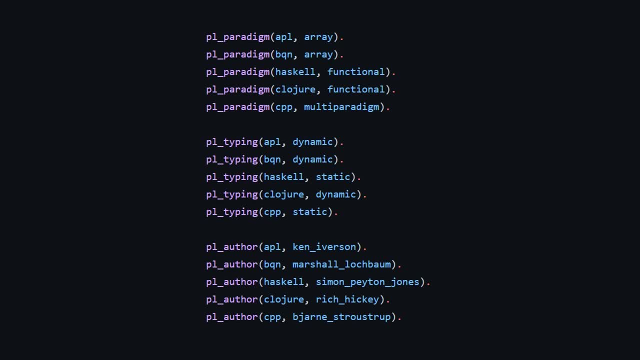 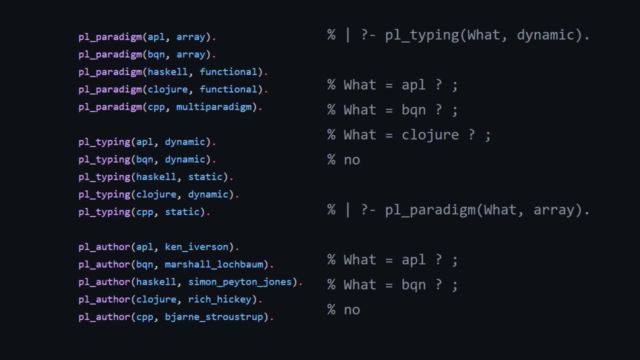 and a multi-paradigm for C++, And then we have some typing information and the authors of these languages And you can query things like how many languages have dynamic typing And when you do that, you get that APL, BQN and Clojure and how many languages are in the array paradigm And you 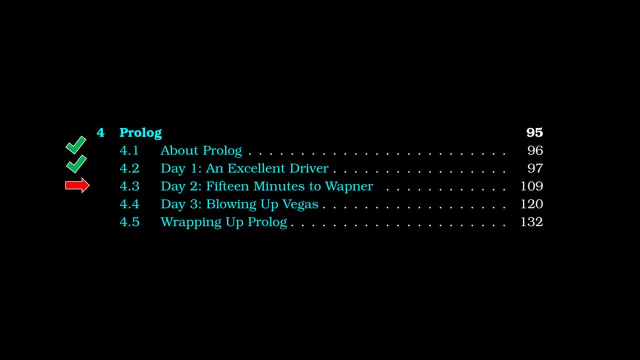 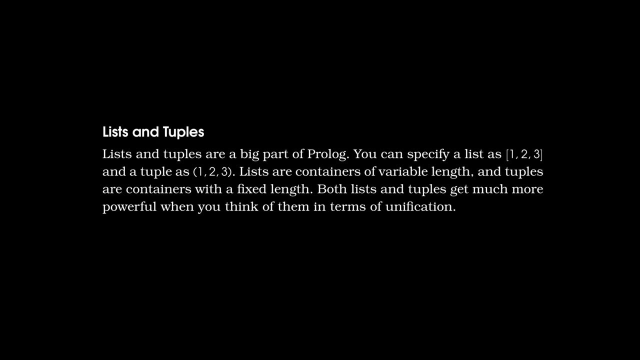 get back APL and BQN, So pretty cool. Moving on to day two, here they start to introduce some more facilities in the language. Lists and tuples are a big part of Prologue and they're going to be used in Prologue. You can specify a list as bracket 1,, 2, 3, and tuples as parentheses 1,, 2, 3.. 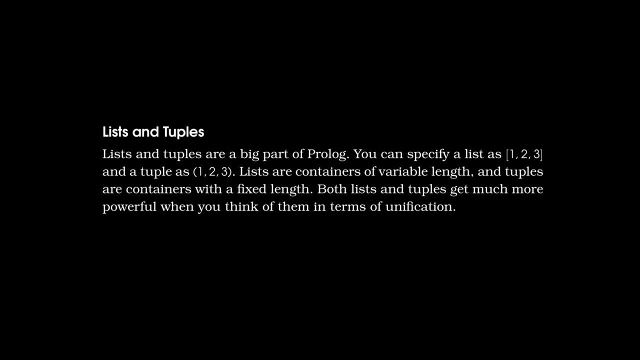 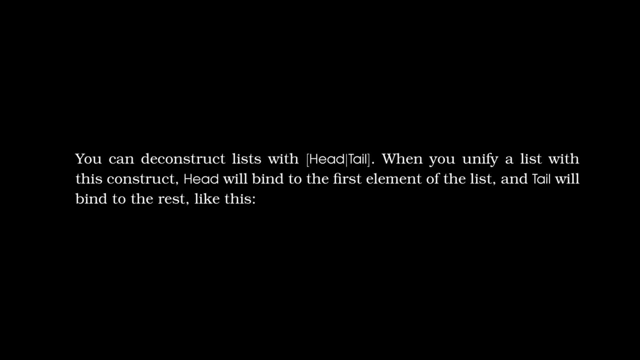 Lists are containers of variable length and tuples are containers with a fixed length. Both lists and tuples get much more powerful when you think of them in terms of unification. And it also mentions in the text- and this is very important for sort of recursion: you can deconstruct lists with head. 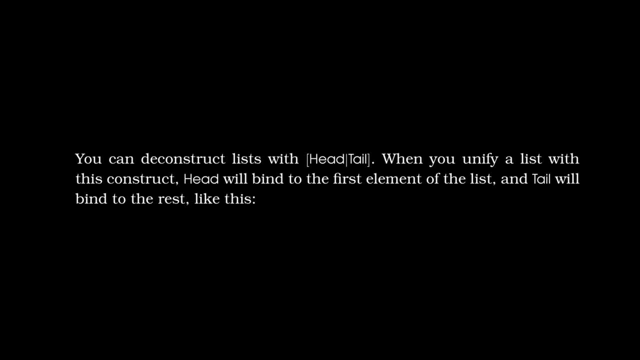 with bracket: head, pipe, tail and bracket. When you unify a list with this construct, head will bind to the first element of the list and tail will bind to the rest, as follows- And note that this is very similar to other functional languages. The first one that comes: 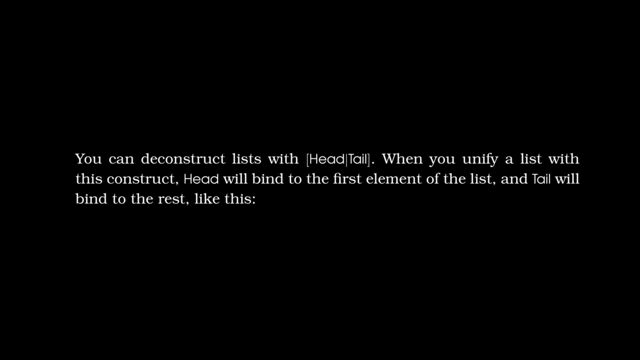 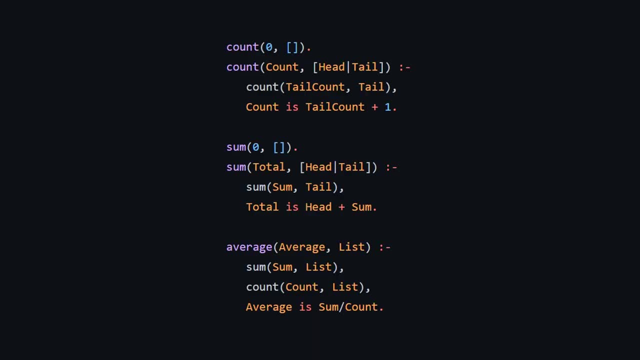 to mind is Elixir, and that makes sense because Prologue influenced Erlang, which influenced Elixir, But there's other functional languages that have pattern matching that work like this as well. Taking a look at the next example which comes from the textbook, and this is basically: 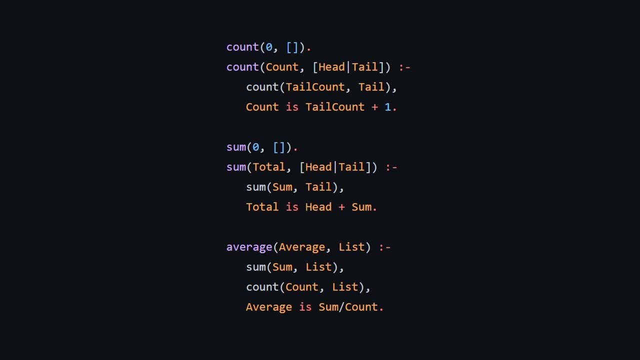 counting, summing and averaging. So you can see here I'm not going to go through this in great detail, but we're using recursion for all of these And we start off with a base case where you have an empty list for both count and sum and that's equal to zero. 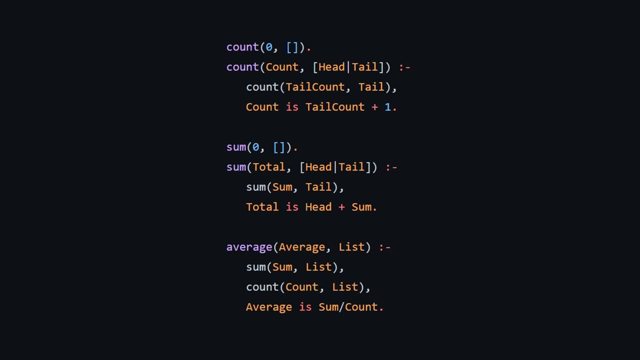 And then, when you are counting, you're basically your first assertion inside your rule is going to be the recursive call to tail, count and tail, and then you're performing the operation in order to do your reduction in the form of adding one for each of your counts. Note: 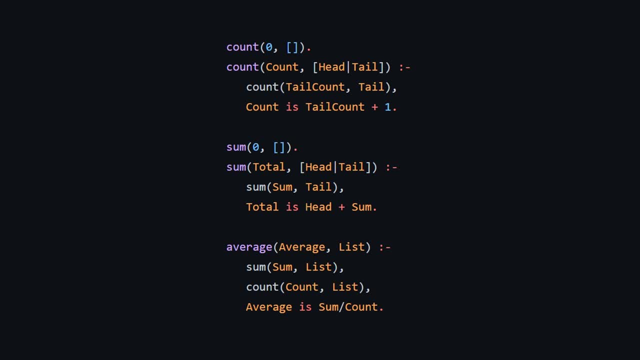 that the comma that separates sort of the recursion call and the reduction call, that represents or, And we'll reflect on that a little bit later as well. So some does something very similar. So the first assertion of doing a plus one is doing a plus sum and average, basically. 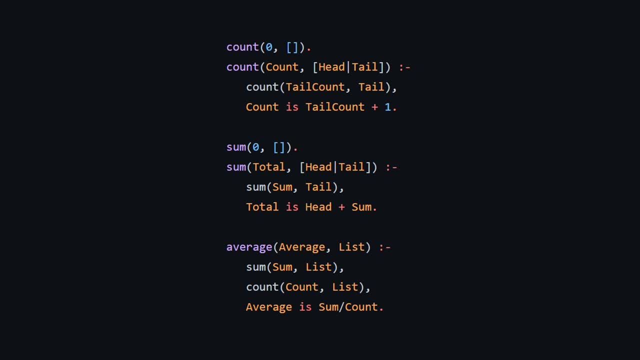 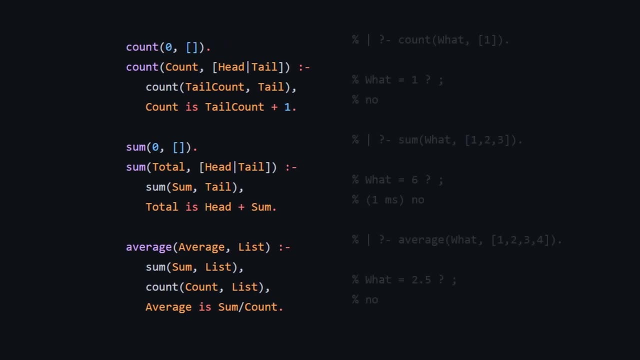 doesn't do any recursion. It's just basically going to make two calls to sum and count and then say that average is the sum divided by the count, which should hopefully be pretty clear, And when you have this all set up, you can do a bunch of different queries. So you can. 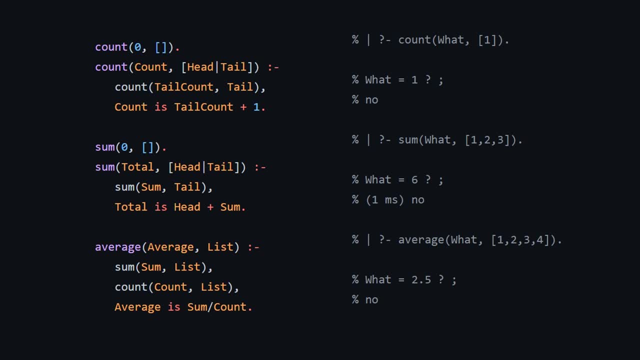 count how many elements are in a list of one element, You get back one. You can do a query where you're summing what is the sum of the list: one, two, three, which is six, And if you do average of one, two, three, four, you get back 2.5. 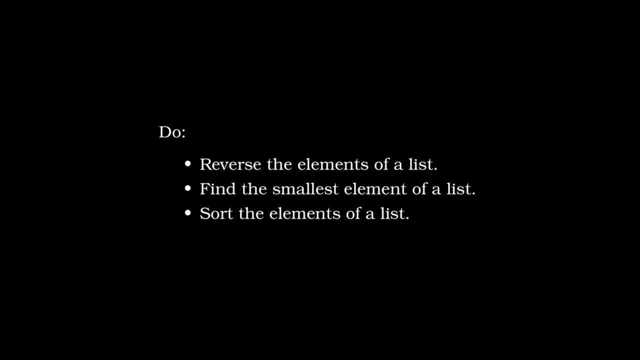 And this brings us to the exercises for day two, which is reverse the elements of a list, find the smallest element of a list and sort the elements of a list. So I actually found these pretty difficult to solve based on what had been introduced. 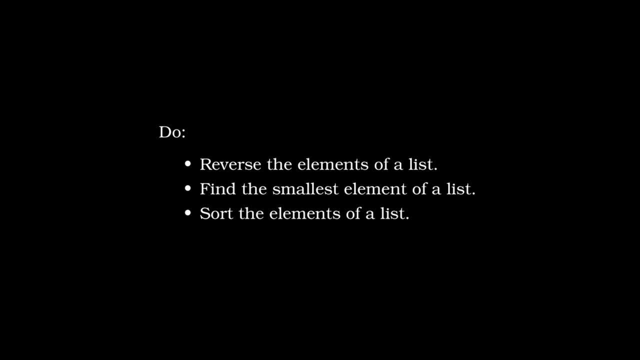 so far. in days one and two I had to Google basically for all three of these solutions. At one point I was able to implement my own sort without having to go Googling, But the first two solutions for reversing and finding the smallest element- both use this sort of 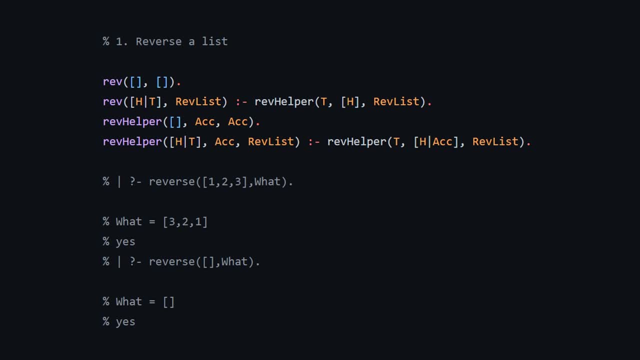 pattern of setting up a helper function with an accumulator, which is very similar to how you might have solved this if you followed along for the structure and interpretation of computer programs and scheme when we were building up reduction functions or algorithms. And it's pretty straightforward, once you see this pattern, that we basically have an accumulator. 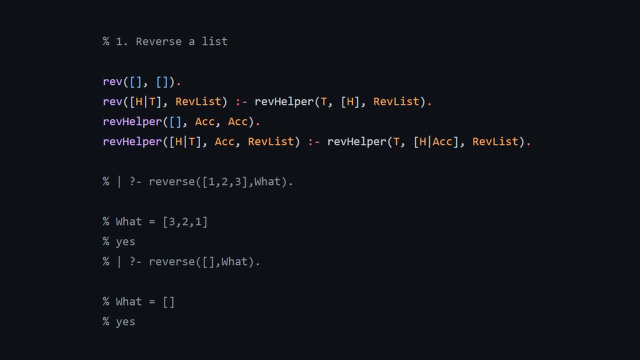 for the reverse helper, that is, the reversed list for each iteration, And when we go through the minimum, it'll be the minimum so far. But without having seen this pattern, I'm not exactly sure How Bruce was expecting us to solve this, And it'll be interesting to see other solutions. 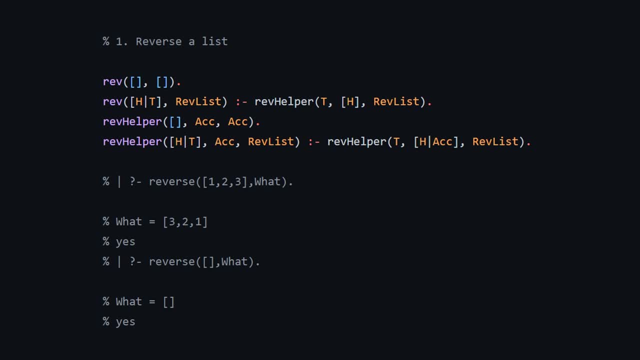 when the meetup takes place. But basically, once you have this helper function set up, you're able to define rev. Note that you have to use something different than reverse, because reverse is a built-in function for gprolog, the version that we're using with this textbook. 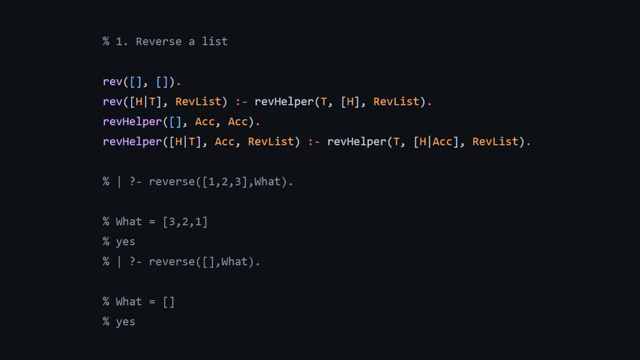 And once we have that set up, we can do reverse 1,, 2,, 3, and then what? And that's going to give us back 3,, 2,, 1.. And if you reverse the empty list, which is a good unit test case, 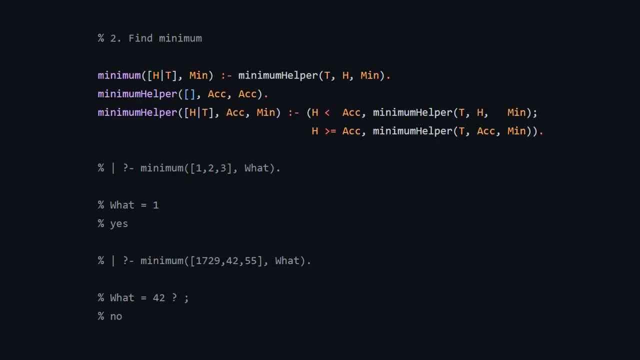 it's going to just return you the empty list Moving on to the minimum, which is sort of very similar to the reverse, The only difference being sort of in the minimum helper. instead of building up a reverse list, we have this somewhat complicated expression. that's basically saying if our current element is less than 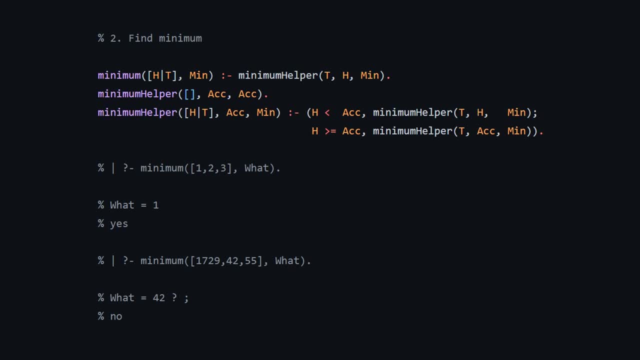 our accumulator, then store that as the minimum now. Otherwise, if it's greater than or equal to just use the current accumulator And note that here the semicolon that we see in the midst of the two parentheses where we have the less than and the less equal to. 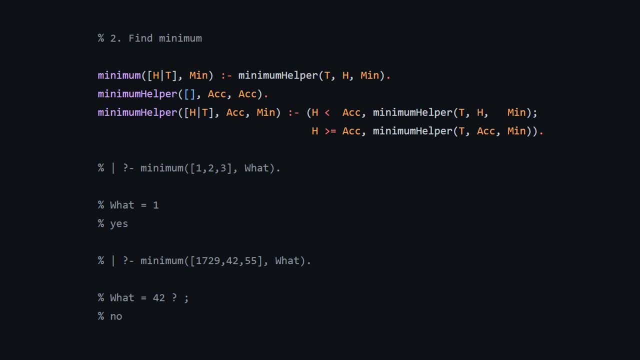 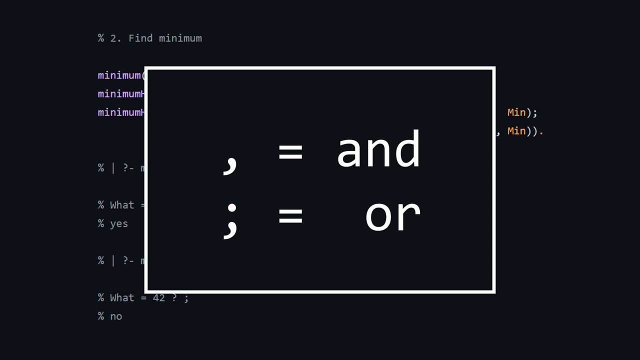 right over here. that is the logical, and So note that I mentioned before that comma equals or- sorry, logical or- Comma equals and, and semicolon equals or. And this is actually something that's not covered in the textbook, which I find pretty unfortunate because it 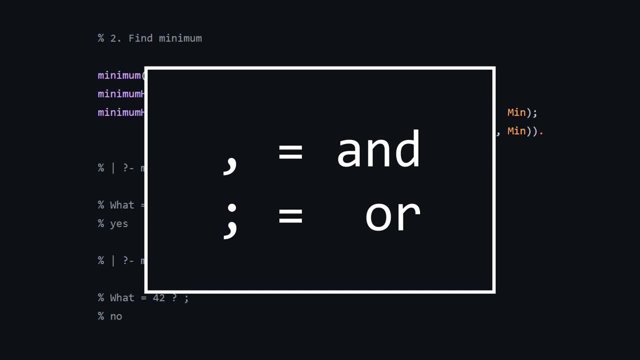 seems like a pretty fundamental thing. So note that when you're building up these sort of rules, comma means and, and semicolon means or, And there's also syntax for sort of if, else I don't think that gets introduced either, but you don't technically need it to solve. 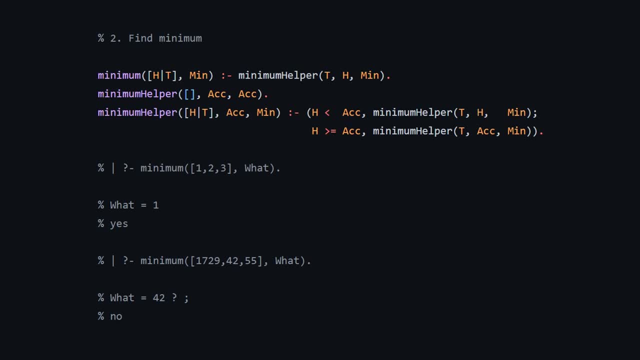 these solutions. That out of the way, once we have this built up, you can do the minimum of the list- one, two, three and you get back one- and the minimum of 17,, 29,, 42 and 55 and. 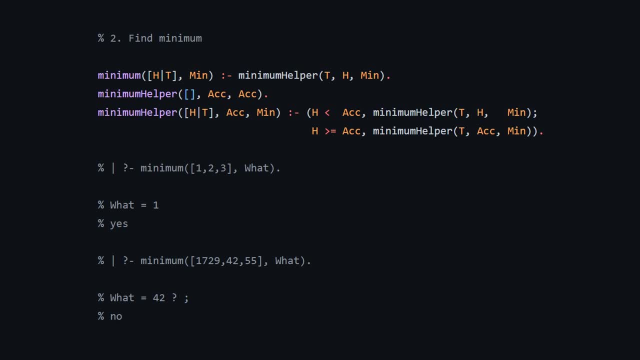 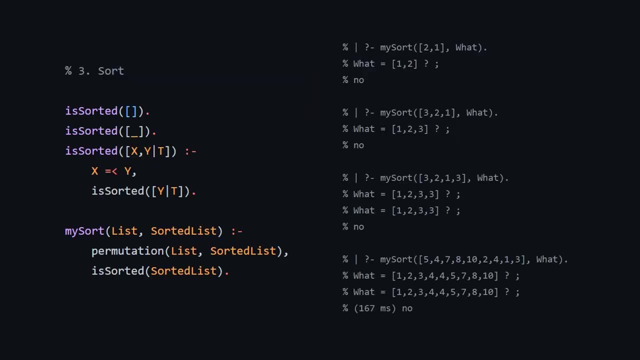 you get back 42.. And last but not least, for day two, we have sort. This is the final solution that I ended up writing, and it basically makes use of a built in function called permutation. I'd be interested to see a solution that doesn't use permutation, but you have this top level. 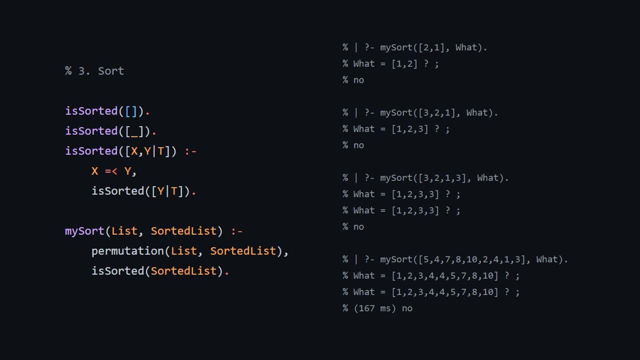 function- my sort that basically makes has two requirements: that your sorted list is a permutation of your Original list and that the sorted list is sorted. and is sorted is pretty simple to define recursively. You basically just check that the element X is less than or equal to Y and 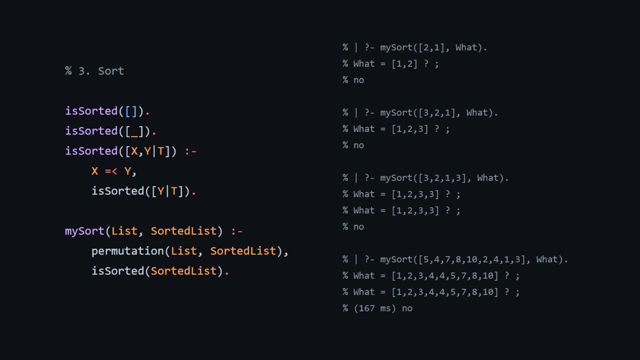 that the you know, when we're looking at the two elements at the front of the list that you currently have, the one on the left is less than or equal to the one on the right, and that the tail of that list, which is basically Y, combined with the tail after destructuring. 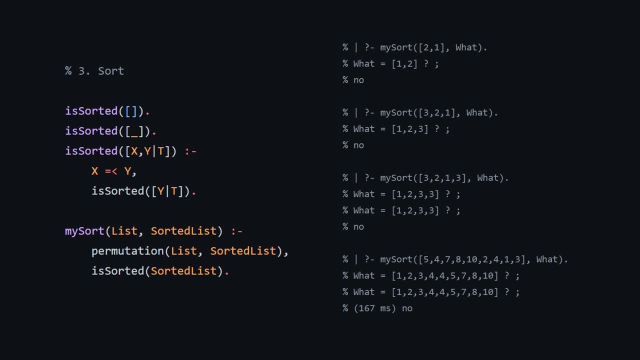 it is also sorted. So this is going to be very, very inefficient, but it does work And I thought it was the simplest sort of solution to solve. This is kind of naively sorting in prologue. There are much more efficient ways to do this And, last but not least, moving. 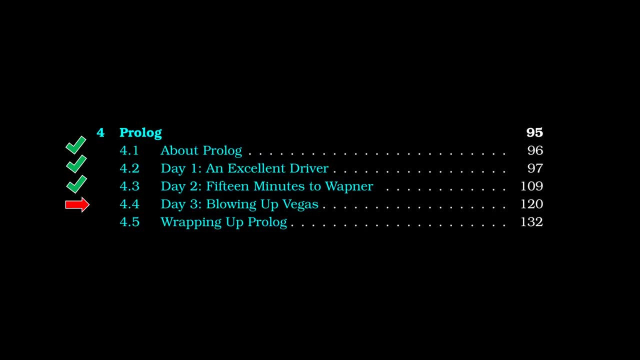 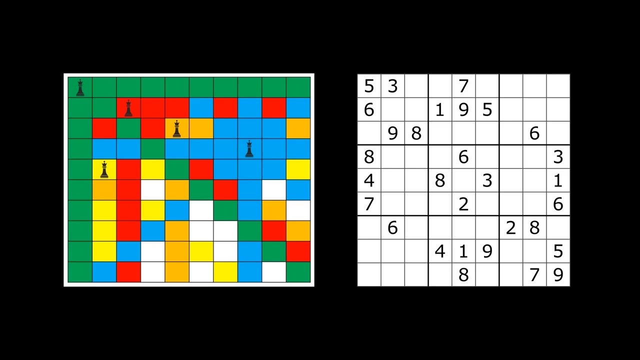 to sort of the most significant day of the three days, day three, And this basically this day we cover two different problems in the book. The first one is eight Queens and the second one is solving a Sudoku. So we're going to go through these pretty quickly. 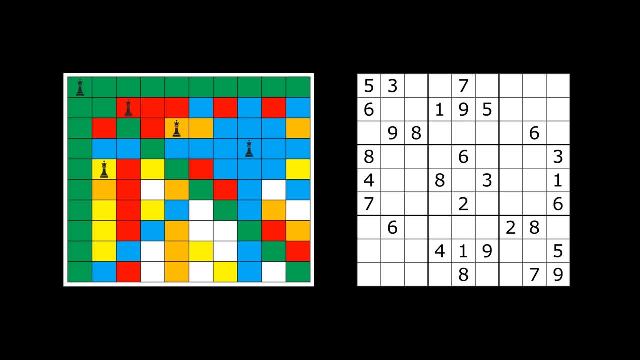 but I encourage you to read through this whole chapter, where it goes into this in more detail. Eight Queens is a pretty famous problem, And actually I covered a variant of this problem In a top coder solution video that I made, I think, in 2018, so almost four years ago. 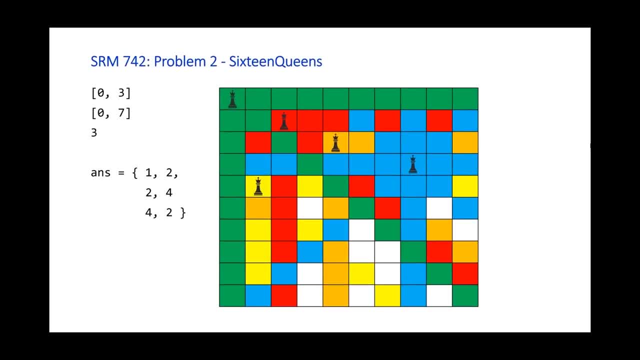 I will leave a link in the description and you can click on the top right If you want to go watch it. note that this was Connor four years ago, So the quality of this video might not have aged well, but the colorization is quite nice. So it shows that you're placing 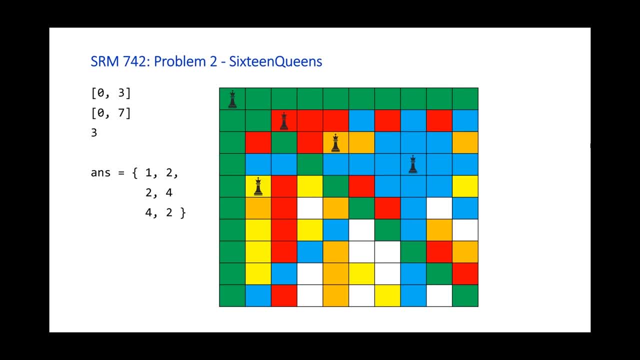 a queen and then you can't place the next queen on any of the spaces where a queen can move to, which is basically vertical, horizontal and diagonal. So the next place you place a queen here is on the red tile, and then that gets rid of. 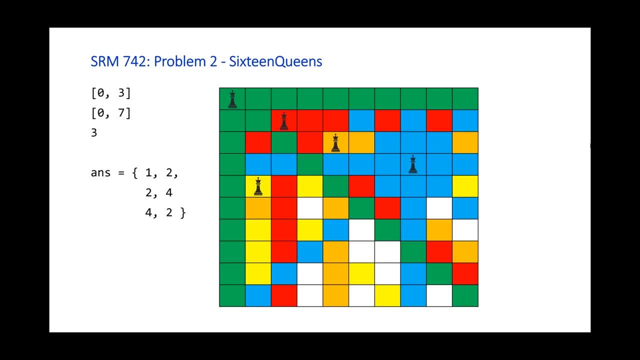 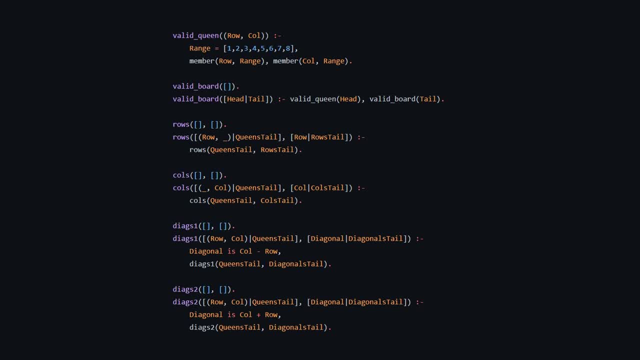 some more ones And then you keep going, which is sort of just demonstrated by the blue, the yellow and the orange and the code that you use to solve this. Like I said, we're not going to go through this in a lot of detail, but it's basically doing the same thing. that. 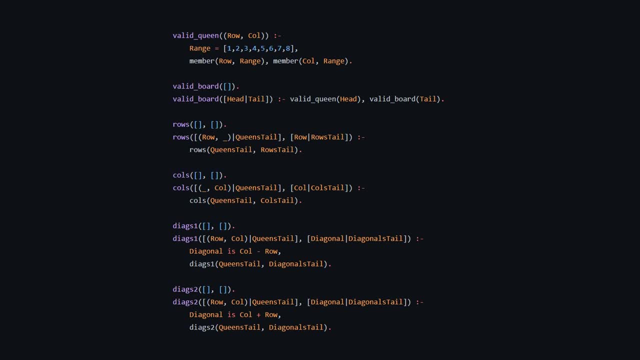 the visualization just showed for rows, columns and diagonals. And once you've placed something you want to make sure that none of the other future Queens are going to be in those spots. And once you have all of this, these helper functions set up, you basically can define. 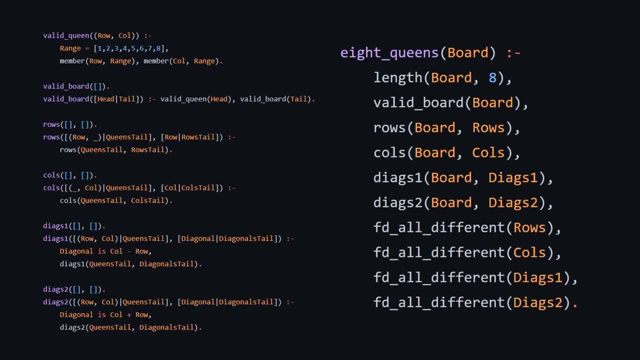 an eight Queens, A solution that defines the length of the board, says the board is valid, and then sets up the rows, columns and diagonals and make sure that all of those are different, which is this built-in G prolog function, FD- all different. So, uh, pretty straightforward. 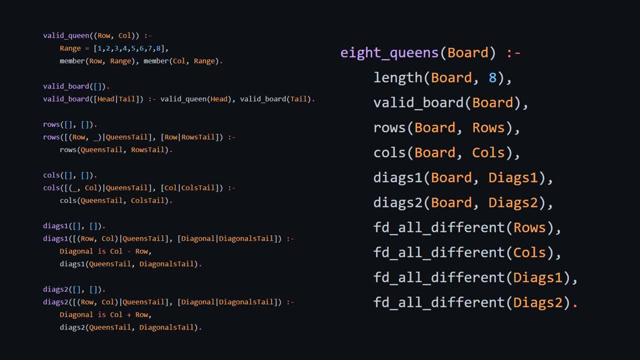 to solve. You don't really need to work through any of the looping or, um, you know, nested for loops in order to traverse the board and make sure that the spot isn't already taken. Pretty neat And last but not least, is the Sudoku solution. This one is actually very 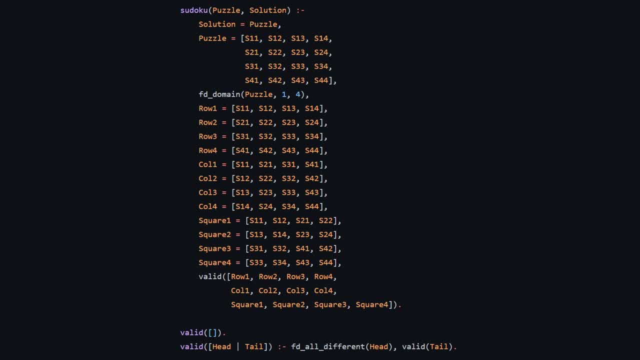 trivial. I'm not sure if there's a nicer way to do this, but they show this in the textbook as sort of the naive way to solve this. You build up a solution and a puzzle and you basically pencil in, and this is just for a four by. 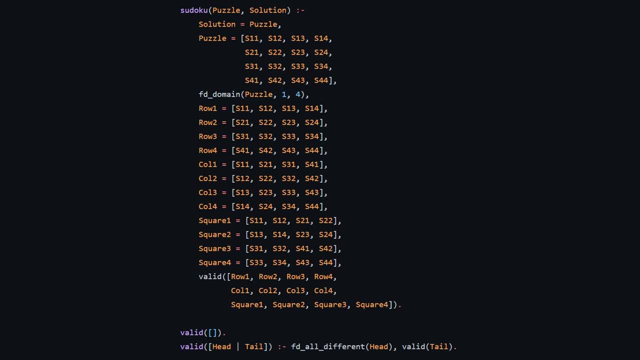 four Sudoku puzzle, not a full nine by nine. You pencil in each of the spots, So you know: spot one one, spot one two, et cetera, all the way to spot four, four. Then you define rows, columns and squares where you have to make sure that all of the values in a row 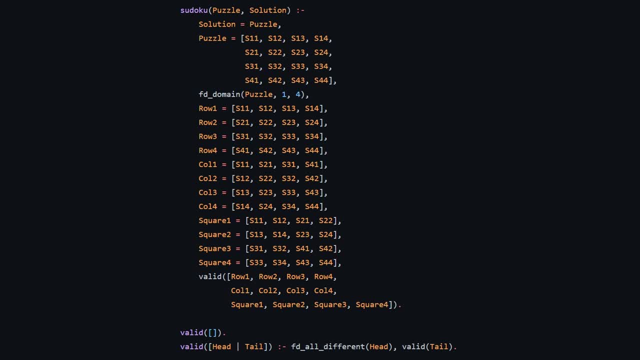 a column and a square are different And then you basically do something very similar to what we did in the eight Queens, Probably a little bit different than what we did in the column. You can see we have the F, D all different uh function at the end And once 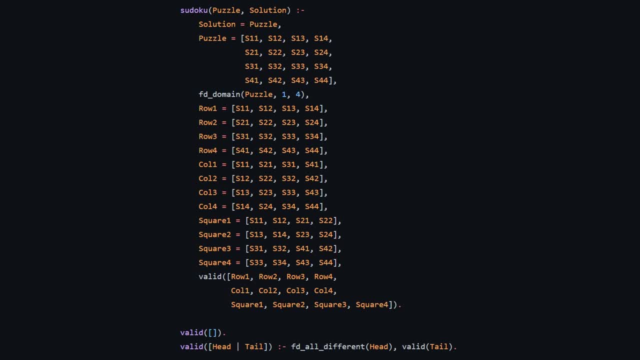 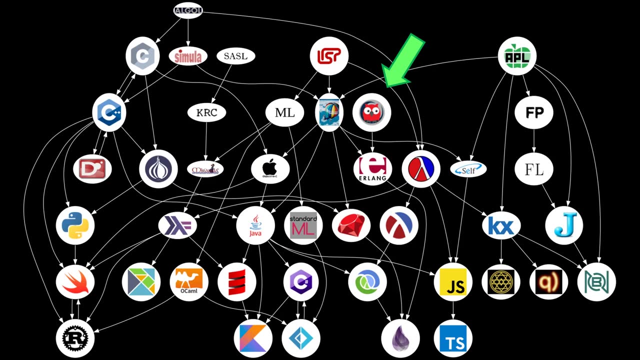 you've done this, it'll solve, which is pretty, pretty amazing, if you ask me. So, all of that being said, that is our summary for the prologue chapter. I personally was not a big fan of prologue. This seems less like a programming language and more like a constraint solving. 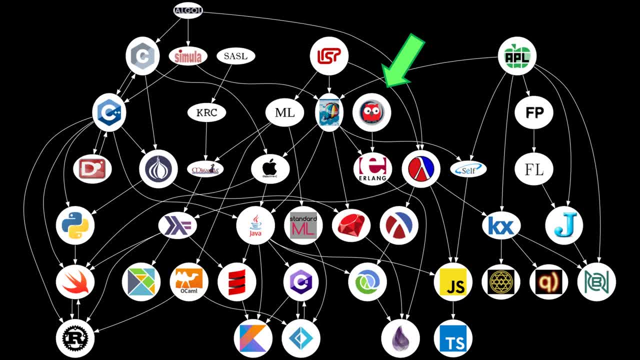 system And I also found it very non-trivial to solve some of the problems at based on where we were at in the book. Like I said, the semicolon hadn't been introduced, Uh, the sort of iterative, uh helper function pattern hadn't been introduced. 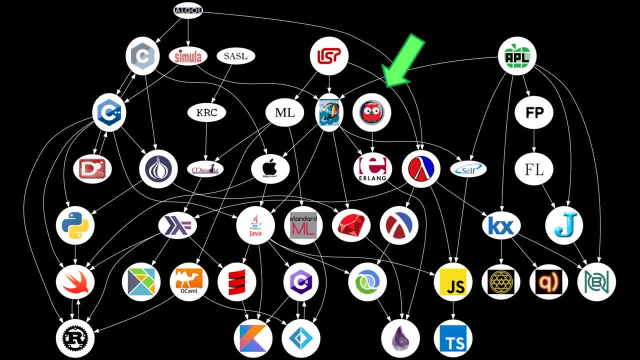 So hopefully we'll get some more submissions before the meetup happens in a couple of days and we'll get to see how other people solve these Cause. uh, admittedly I had some difficulty. It would definitely wasn't as easy as IO or Ruby, but I did have previous Ruby experience. 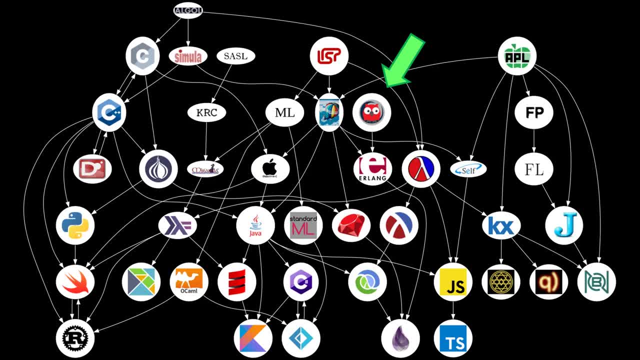 So maybe it's just that I was more familiar with the other paradigms than the logic programming paradigm. That being said, I hope you enjoyed, I hope you learned something and we will see you in the next chapter, In the next video.